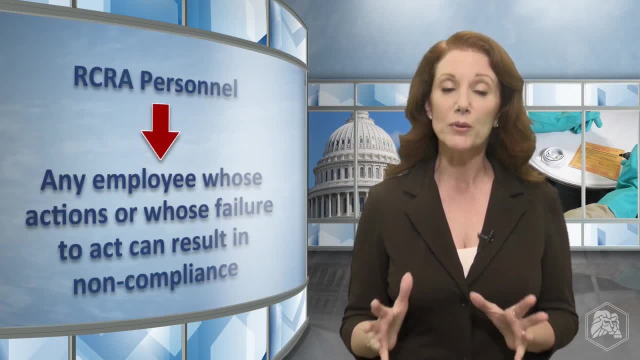 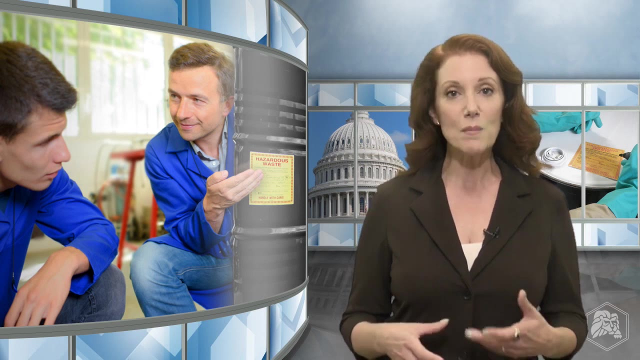 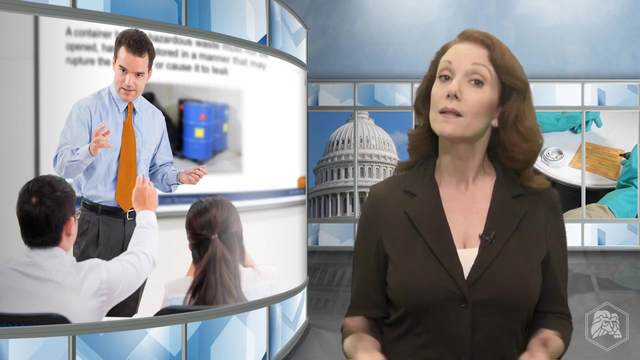 The EPA defines RCRA personnel as any employee whose actions or whose failure to act can result in non-compliance. RCRA training must teach personnel how to do their jobs in a way that maintains compliance with the EPA's hazardous waste rules. This training must be led by someone trained in hazardous waste management like a Lion. 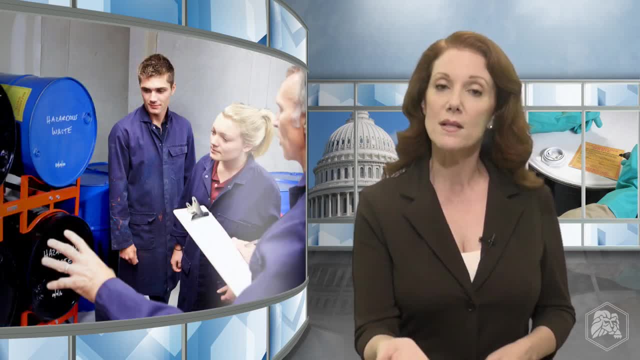 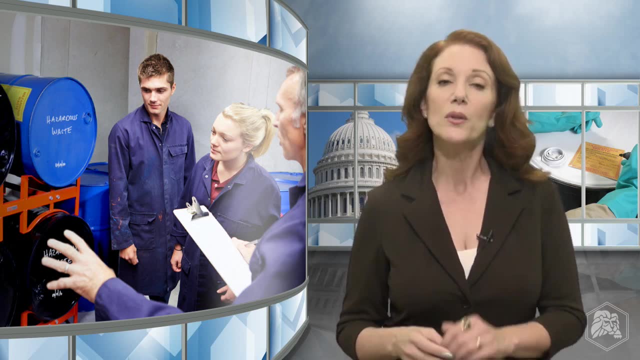 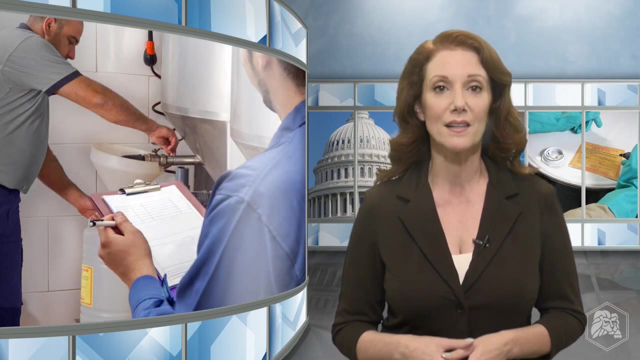 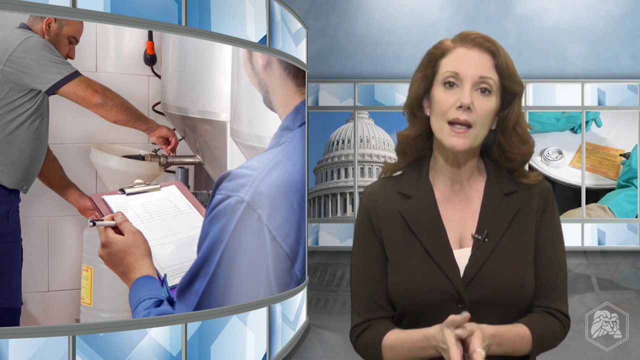 technology instructor For new employees at large-quantity generator sites. training must be completed within six months of the date the employee is hired. Until they are trained, new employees must be directly supervised while working at the facility. After initial training, personnel at large-quantity generator sites must repeat training annually. 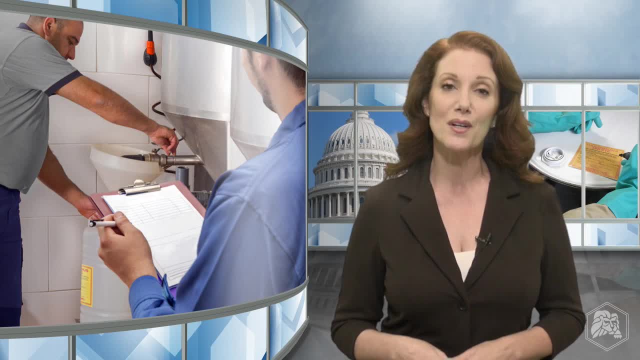 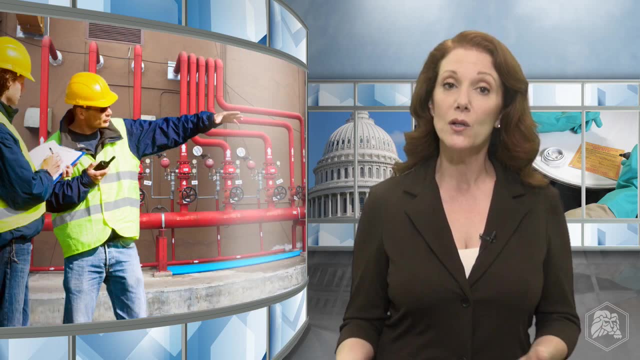 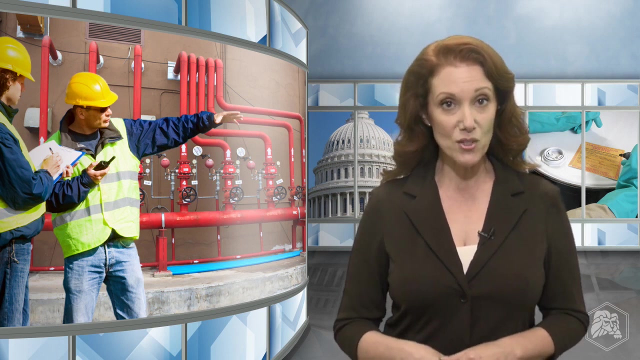 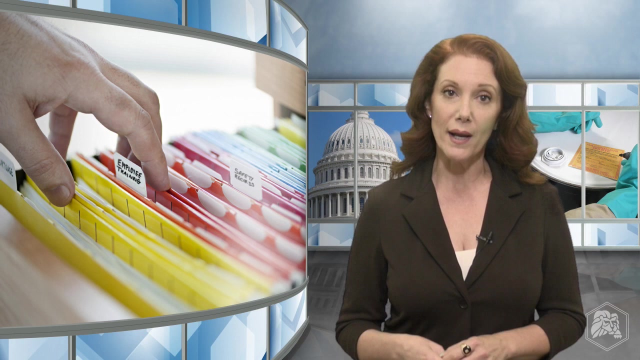 and receive update training when rules change. RCRA training must include some general training, Job and site-specific requirements, like showing employees how to operate emergency equipment, respond to emergencies and even how to shut down operations if necessary. Lastly, large-quantity generators must keep records of training that include the name. 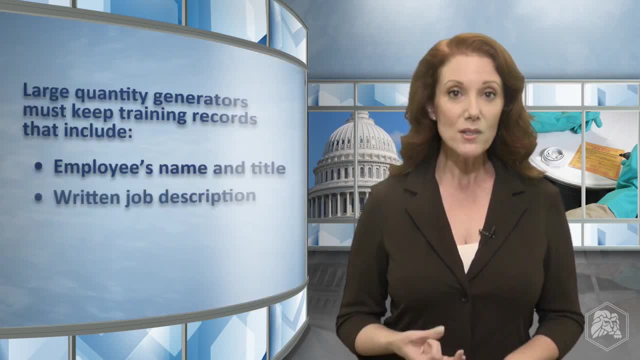 of the employee, the employee's title, a written job description and a description of the type and amount of training provided. The training records must include the name of the employee, the employee's title, a written job description and a description of the type and amount of training provided. 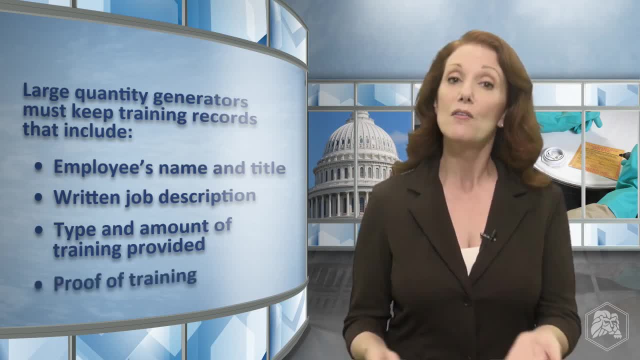 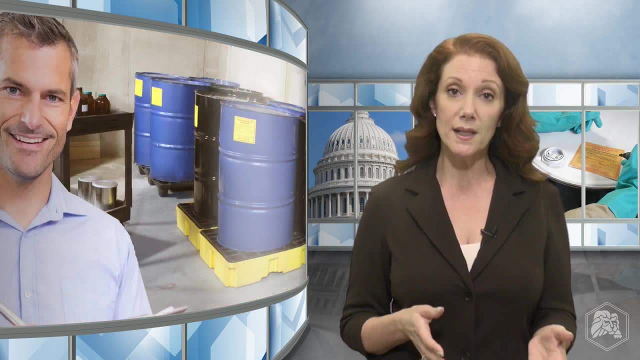 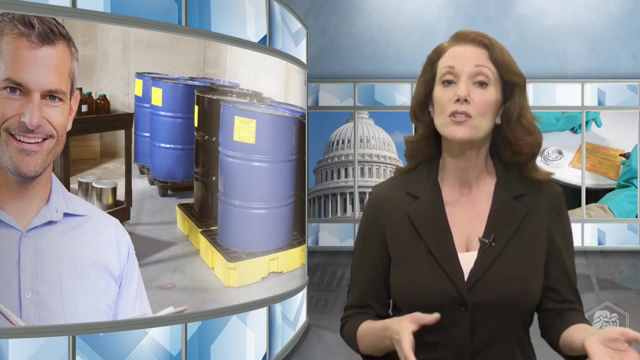 The training record must also include proof that the training was done, for example a Lion technology training certificate. The training requirements for small-quantity and conditionally exempt small-quantity generators are less detailed than the large-quantity requirements we just talked about. 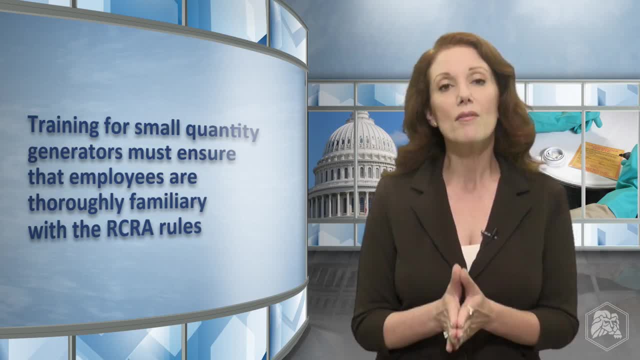 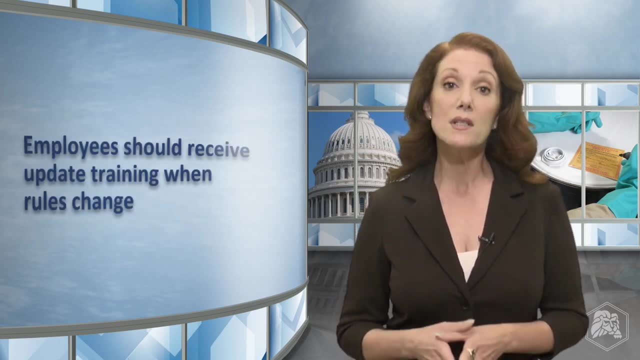 Small-quantity generators must train personnel so that they are thoroughly familiar with the RCRA requirements. When rules change, these personnel should be trained in a similar manner as the training requirements. Employees should receive update training to ensure they remain thoroughly familiar with RCRA. 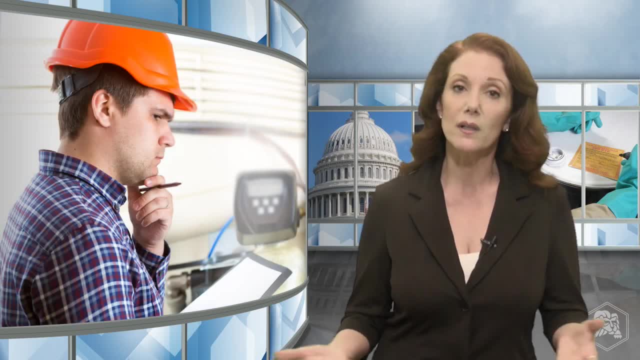 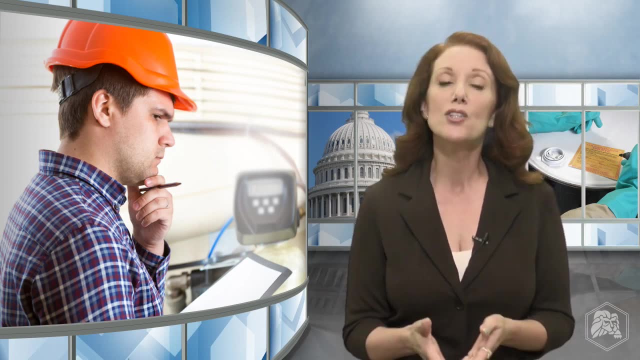 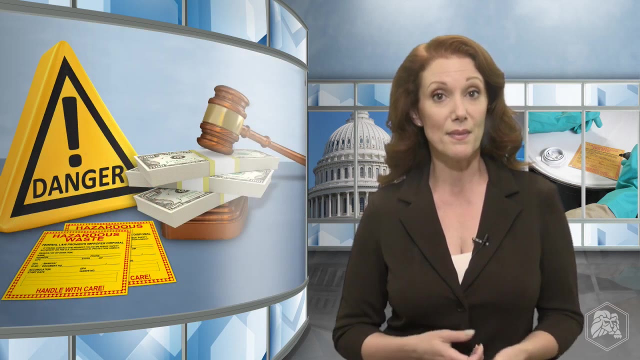 Also, as time passes, personnel may forget critical elements or procedures covered in their training. To keep employees' knowledge fresh and up-to-date, training should be provided at regular intervals. If employees don't know the latest rules, they are likely to violate them putting themselves. 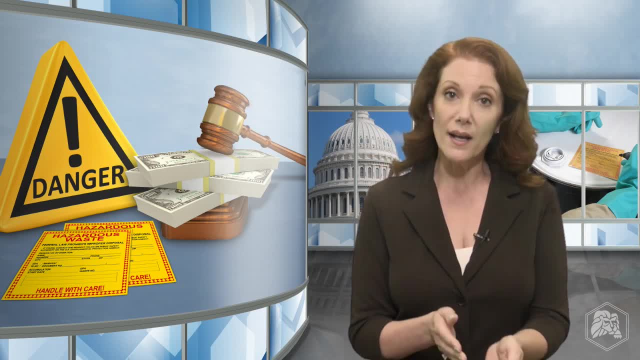 and others in danger and subjecting your site to costly civil law. If employees are not aware of the latest rules, they are likely to violate them, putting themselves and others in danger and subjecting your site to costly civil law. The training requirements must also include the following requirements: